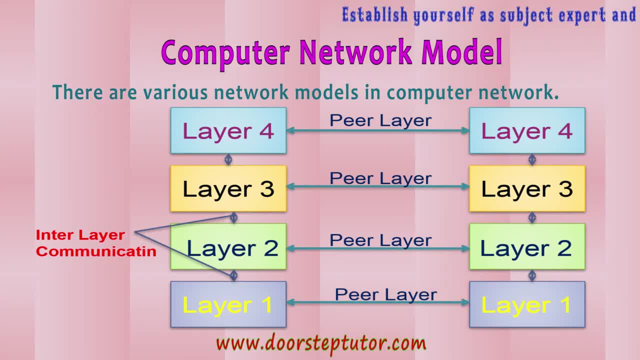 side can inter communicate with each other. also They can send messages, information or anything. depending upon the requirement they can exchange those things. So this is the basic model, how the layered architecture work. There are various network models also available in the computer network which we can use for the transmission of the data from. 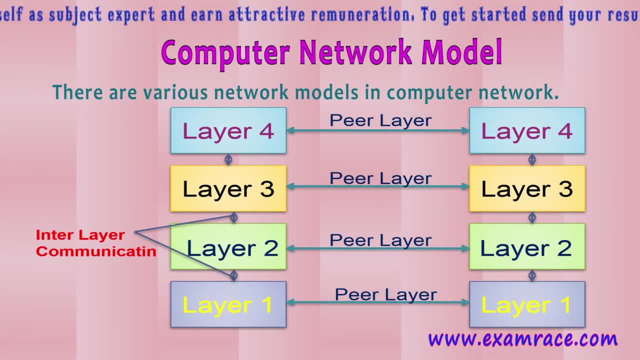 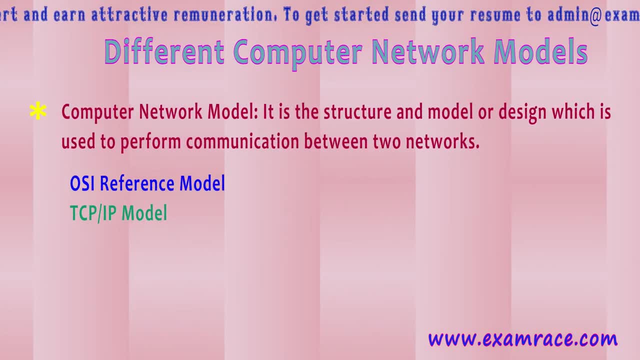 sender to the receiver or we can see that, from source to the destination. So hope this diagram is clear to everyone. Let's move to the second slide, Different computer network models. heard about two most important network models, that is, osi and tcp ip. now let's come to the 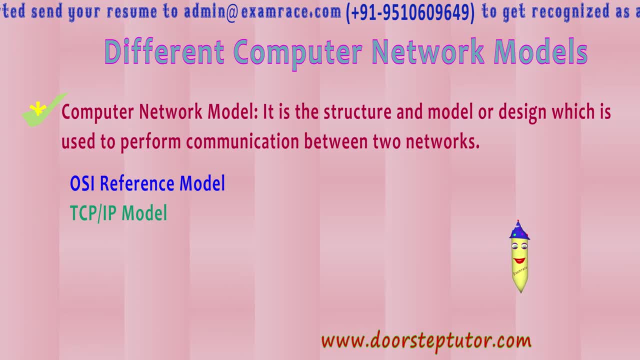 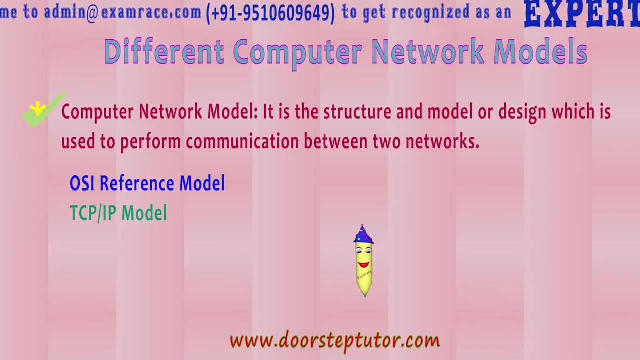 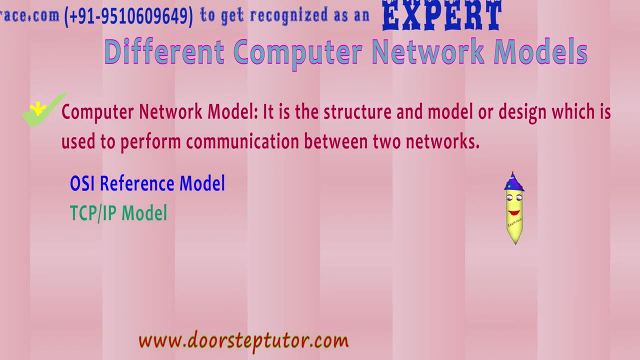 definition of computer network model. first we should understand what is the computer network model. then we will discuss and focus about the different models, like osi and tcp, ip. okay, so what is computer network model? it is the structure and model, or it can be any design which is used. 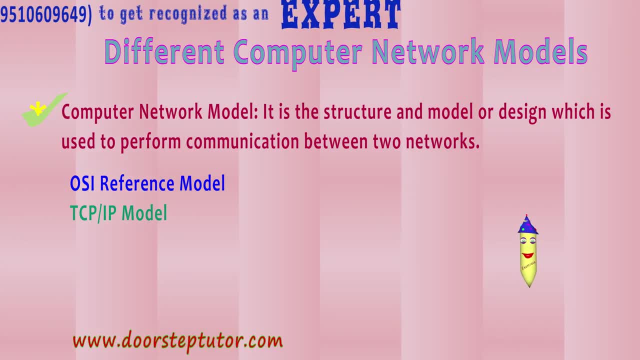 to perform communication between two networks. so if we are having two or more networks, we need to communicate between each other. what we exactly need is model. we should have a structure or a design through which we can communicate easily between the networks according to the requirement. so we are having two types of network models: osi- reference model. osi is usually called as: 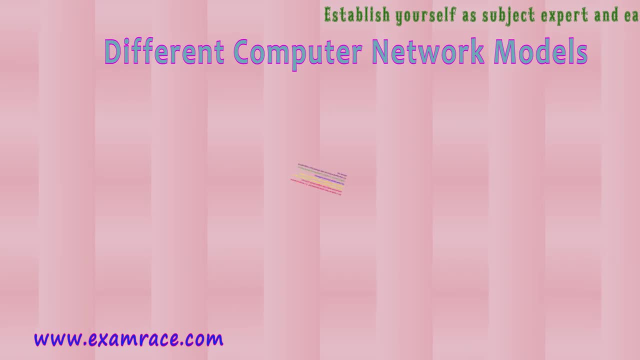 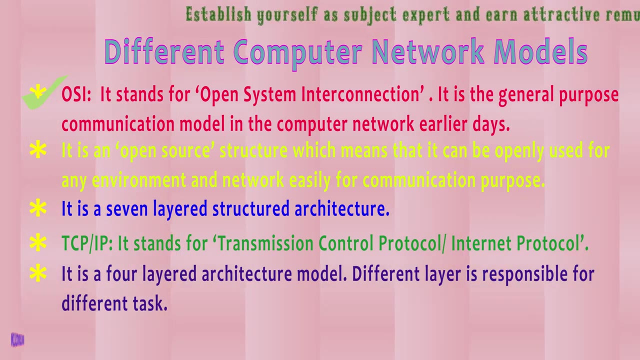 reference model, also osi reference model, so it stands for open system interconnection. this abbreviation is very important. then it is the general purpose communication model in the computer network earlier days. it means that in the earlier days we used to have osi model, but recently we are working on the tcp ip model. 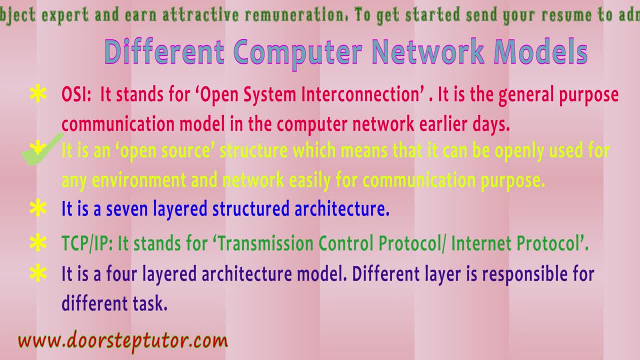 so it has been obsoleted. so the second point under osi is: it is an open source structure. so now, what is open source? open source means that it can be openly used for any environment and network, easily for communication purpose. it means that there can be any other platform or any. 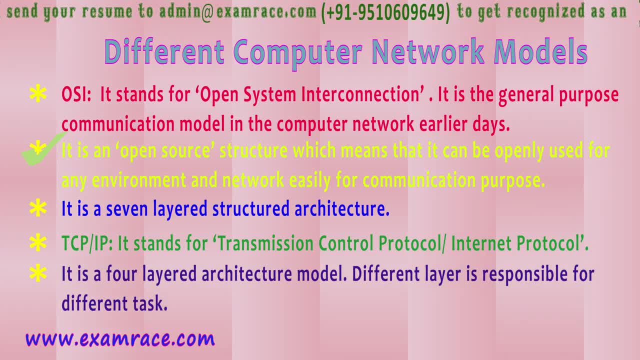 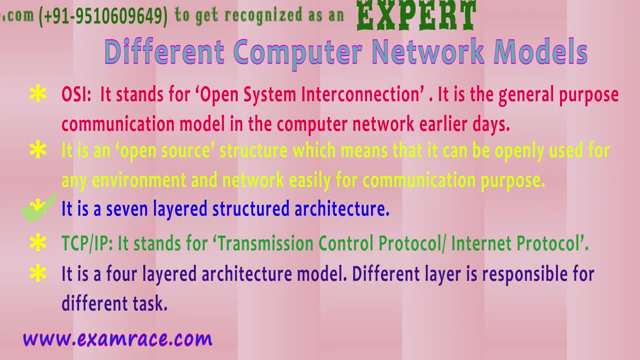 other protocol that is working on the other side. what will happen on the destination side? there will be a compatibility between sender and receiver. so osi is very open source. it is very easy to work in a communication network. so the third point is it is a seven layered structured. 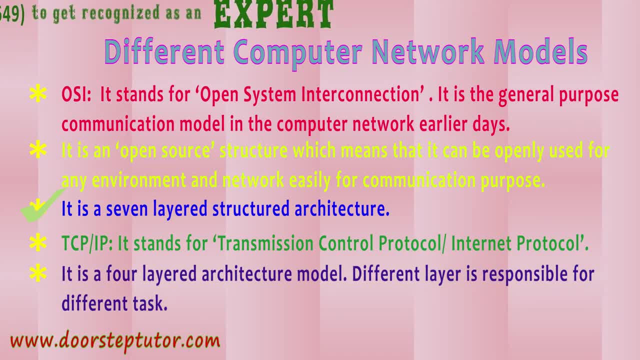 architecture. it means that osi is having seven layers, okay, but the tcp, tcp, ip is having four layers only. so let's come to the second topic, that is, tcp ip. tcp ip stands for transmission control protocol and ip. we know that it stands for internet protocol, full form of tcp ip. then the second point: it is a full four layered. sorry, it is a four layered. 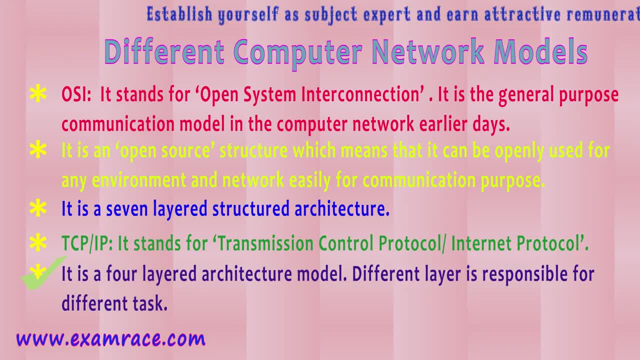 architecture model. different layer is responsible for different task. we can say that if we are having four layers in the tcp ip, every layer will have the individual working and the coordination with the other layers. so this was all about osa and tcp ip. you can go for the detailed information on osa and tcp ip. you can refer other videos also in: 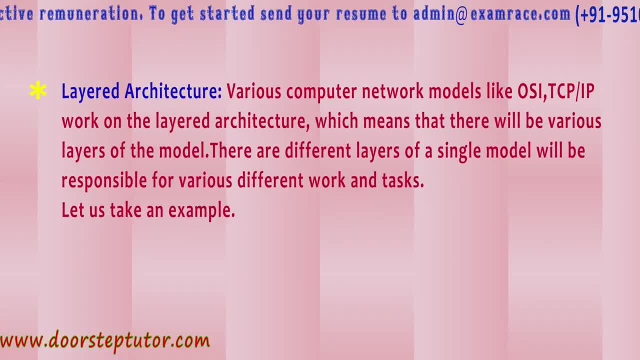 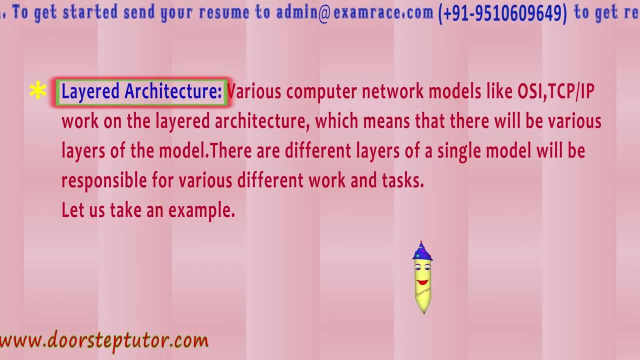 which osa is very explained. so let's move to the next slide, that is layered architecture. so, as its name represents what will be the layered architecture, various computer network models like osa, tcp, ip. they work on the layered architecture, which means the layer architecture is the layer architecture of the architecture of the architecture. 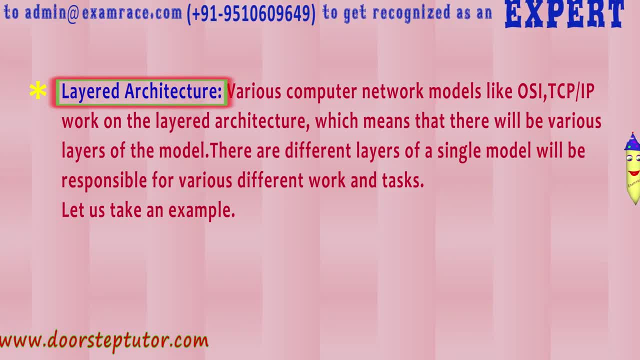 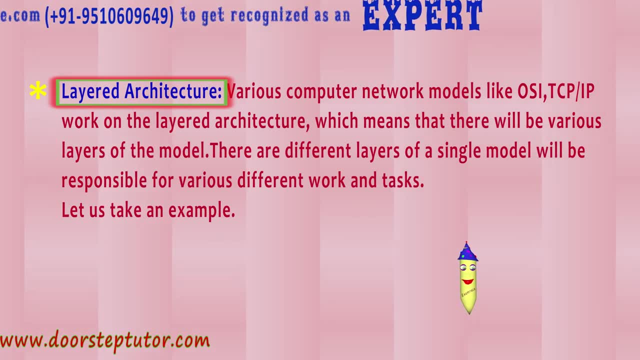 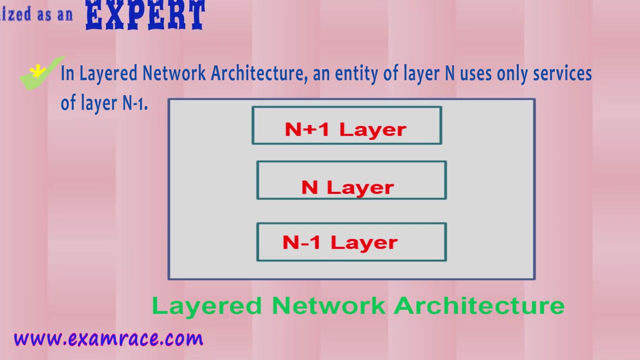 means that every layer in the model is very important. there will be various layers of the model. there are different layers in a single model will be responsible for various different work and tasks. so we can take an example. we can understand the structure in the slide. so we are having n layer at the center, n plus one layer at the top and n. 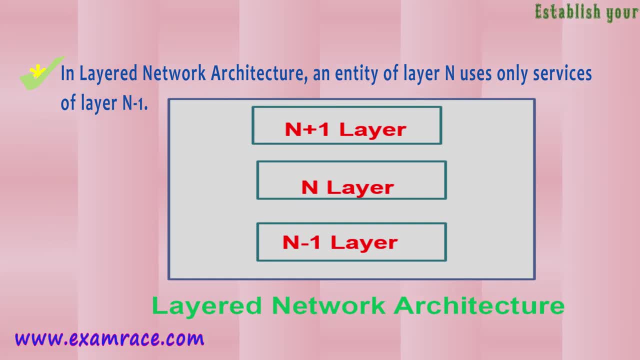 minus one layer at the bottom. it means that every layer in the model is very important. the structure as you see in the slide represents various layers of the inclusiveness we are learning. so the structure ofine every layer of the model is various layers. so it means 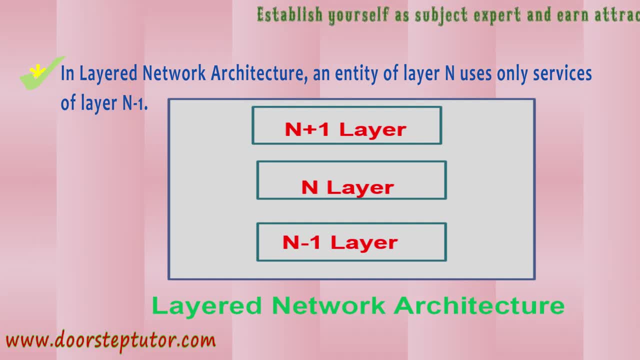 that there will be sequence of layers like ne, layer 1, layer 1, layer 2 layer and lab layer 3, layer 4, and so on, depending upon the transmission protocol on which we are working. so this is the simplest structure and the information will communicated from n1, n minus 1 to n. then 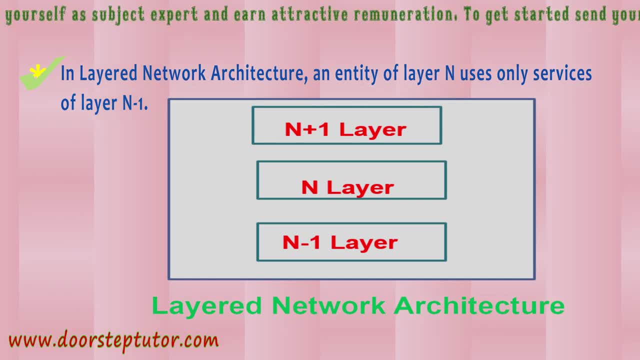 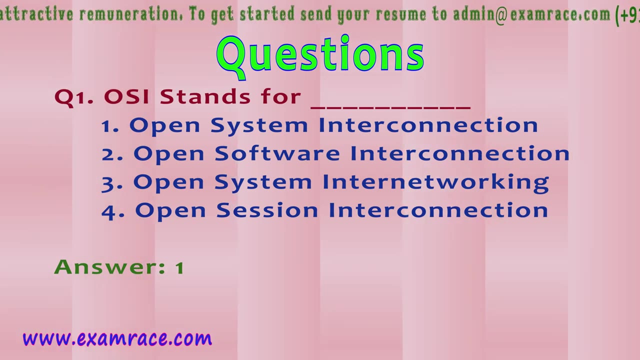 n plus 1, then n plus 2, and so on, and every layer will have the individual function. so this is all about the layered architecture and it's working. so let's move to some of the important questions related to the same topics which we have discussed right now. so first question is: osi stands for? the options are: 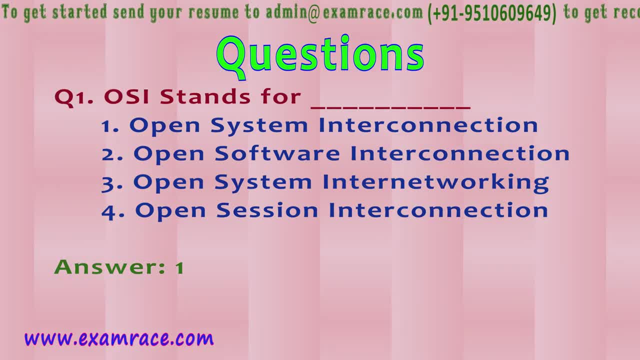 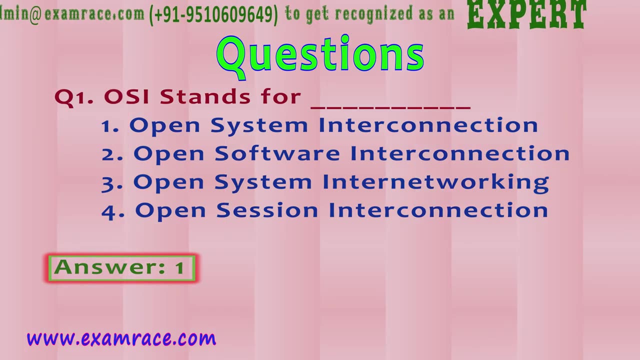 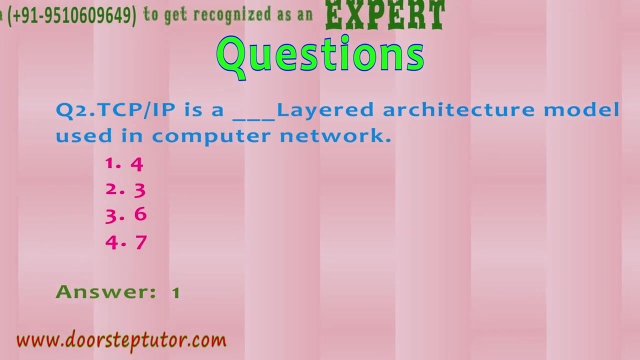 open system interconnection. second option is open software interconnection. third option is open system inter networking. then the fourth option is open session interconnection. so what is the answer? answer is option number one, that is, open system interconnection. let's come to the second question. second question is tcp ip is a dashed architecture model used in. 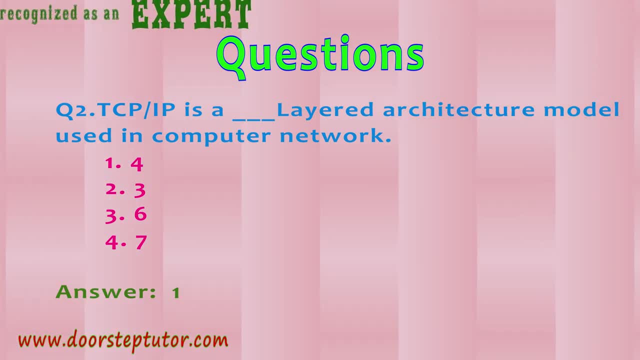 computer network. this is very easy question. so what is the answer? tcp? Answer is option number 1, 4.. TCP, IP, is a 4-layered architecture model. Then the third question, TCP is. So what is the definition of TCP? 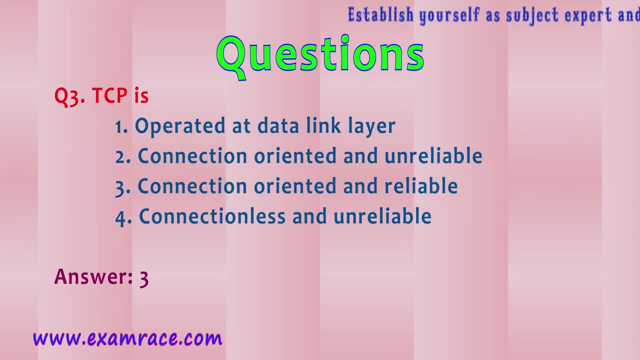 We have to choose for one option from the options given below. The first option is operated at data link layer. Second option is connection oriented and unreliable. Third option is connection oriented and reliable. Then the fourth and the last option is connection less and unreliable. 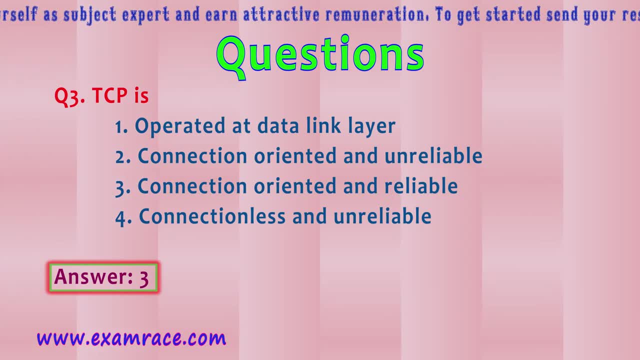 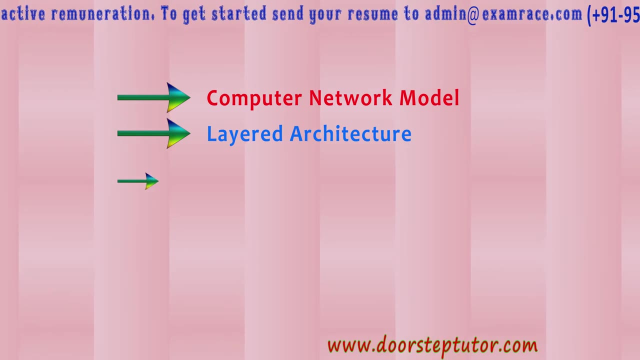 So what will be the answer for this question? TCP is connection oriented and reliable. The option number 3 will be the correct answer. The topics we covered are computer network model, then layered architecture. Third is working of layered architecture. Then we have discussed little about OSI model and TCP IP model. 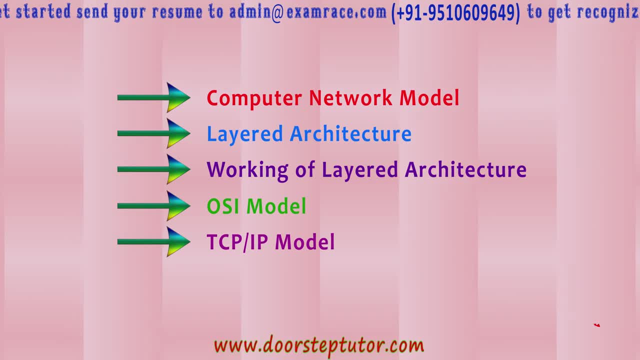 So this was all about the computer network model. Thank you so much.